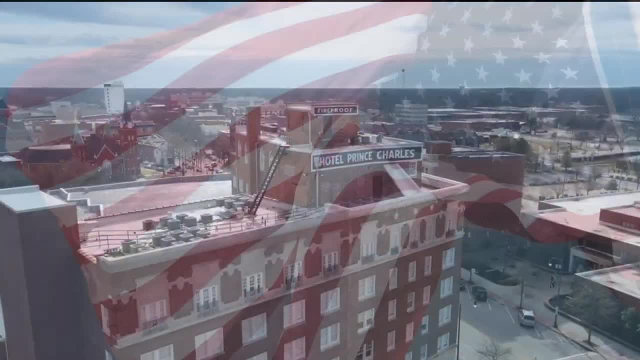 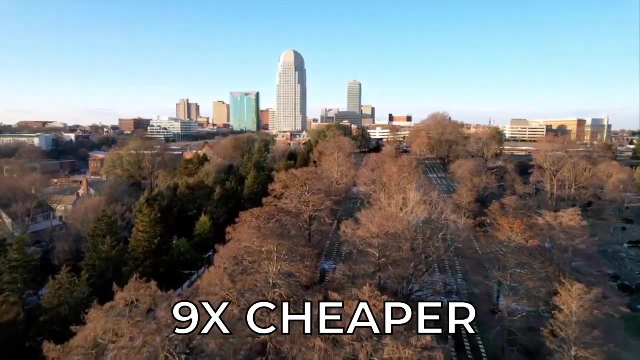 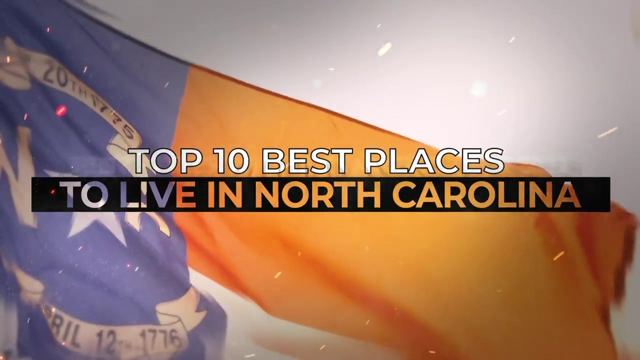 Did you know that Fayetteville has won the All-American City Award three times, or that the cost of living in Winston-Salem is nine times cheaper than most US cities? you know? In today's video, we will be sizing up the 10 best places to live in North Carolina. 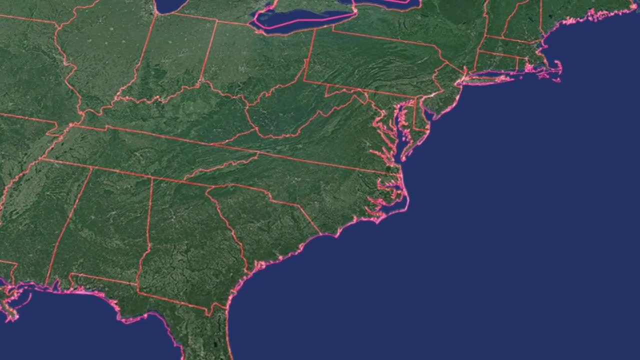 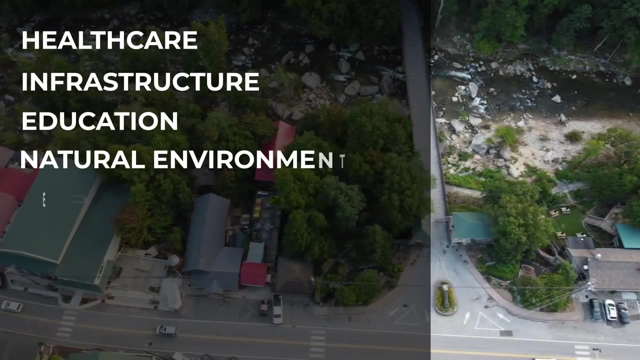 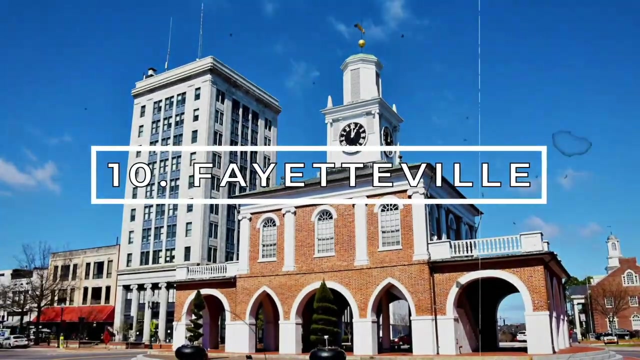 To determine which North Carolinian cities or towns are the most promising, we examined numerous factors, including healthcare, infrastructure, education, natural environment, economy, cost of living, crime rate and more. Here is what we found: 10. Fayetteville, Sitting in the county seat of Cumberland, is 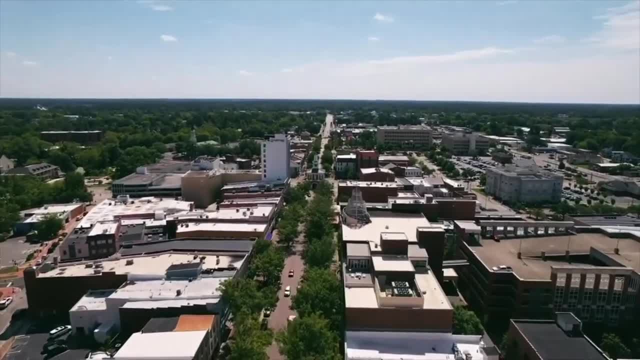 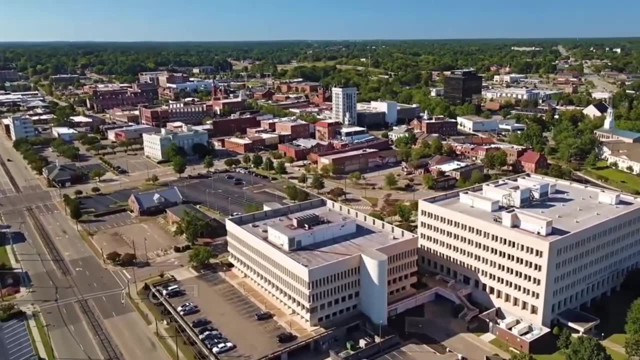 the city of Fayetteville, which is best known as the home of the US Army installation northwest of the city, Fort Bragg. The All-American City has a population of around 210,089 residents. The first thing you see when you enter the city is the city of Fayetteville, which is one of the most popular cities in North Carolina. The city has won the All-American City Award three times. They don't give that to just anybody. Being a military city, people from all over the world move into Fayetteville due to military ties and this gives the city. 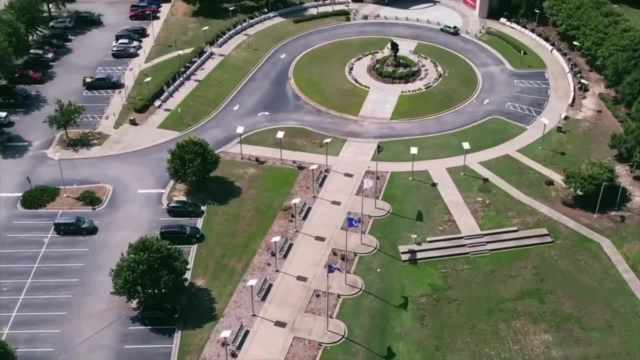 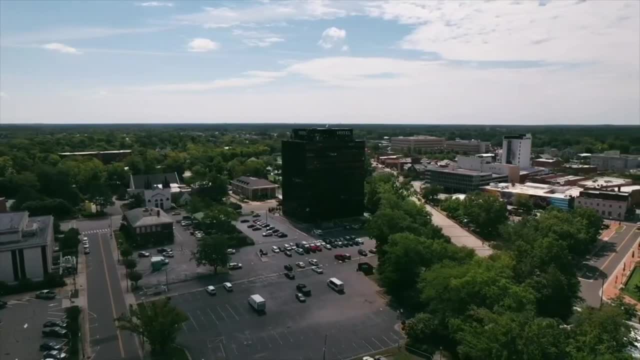 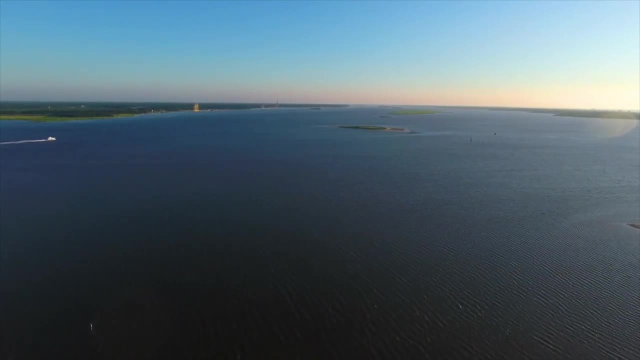 a beautifully diverse culture that anyone would love to be a part of. The All-American City is conveniently located near beaches and mountains, so living here is like a getaway to an exotic resort. Residents and visitors enjoy walks and hikes to the Cape Fear River, while a handful of people take turns paddling down the scenic waterway. While this is very exciting, fun is not the only thing Fayetteville has to offer. The cost of living in the military city is relatively low compared to the state and national average. The cheap cost of living is also reflected in the cost of housing. This means that the 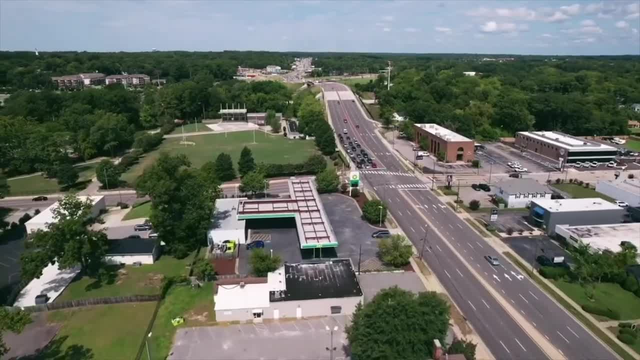 average American can live in Fayetteville without having to pay their way to the military. The cost of living in the military city is relatively low compared to the state and national average. This means that the average American can live in Fayetteville without having to pay their way to the military. 9: Wilmington. Adding a splash to our list of best places to live in the Old North state is the port city of Wilmington, Located in the county seat of New Hanover in the coastal area of southeastern North Carolina. Wilmington is the eighth-most populous city in North Carolina. The port city has a population of about 117,247. 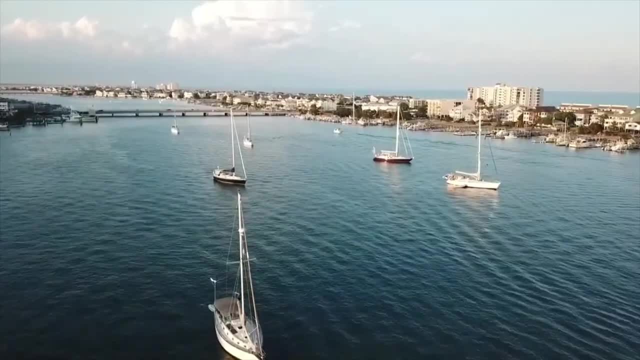 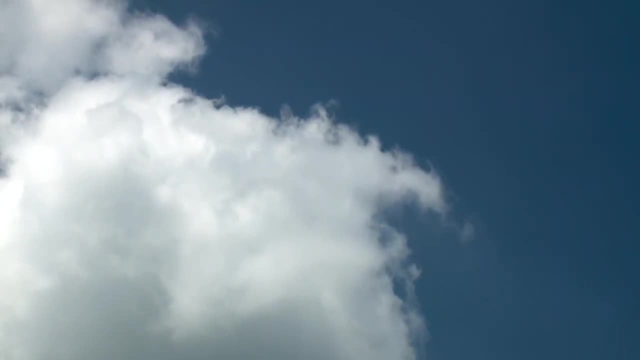 people and a total area of around 50,000 residents. Wilmington is the eighth-most populous city in North Carolina. The port city has a population of about 117,247 people and a total area of 52.9 square miles. The first perk of living in Wilmington is the weather Being so close to the 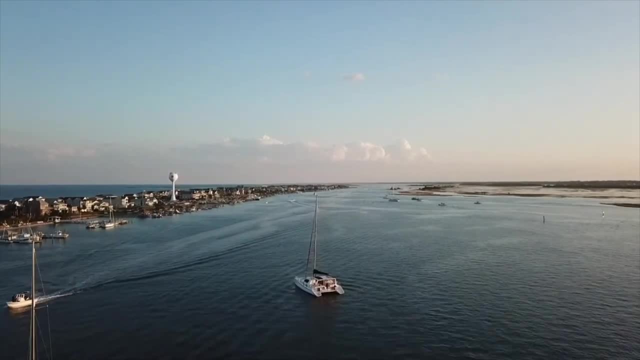 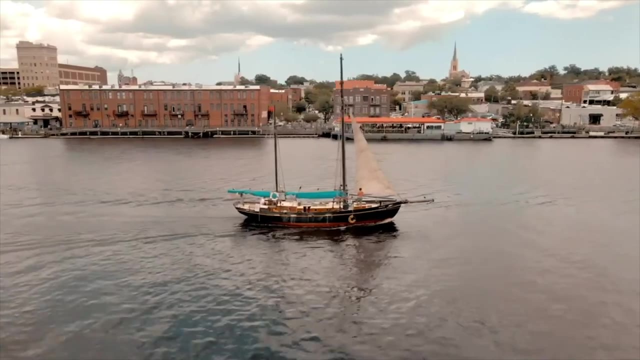 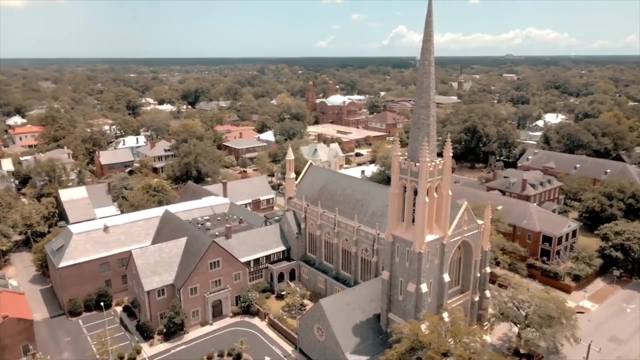 sea. the city has great weather and the cool breeze from the sea is present at nearly all times. Wilmington and its people, like most North Carolinians, value history, and you can see that in every part of the city. The city has several colonial sites that pay homage to the highs and 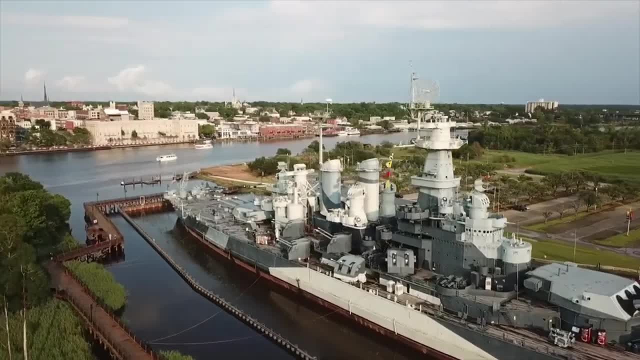 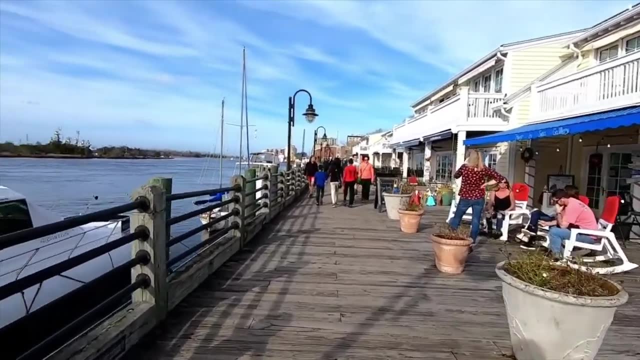 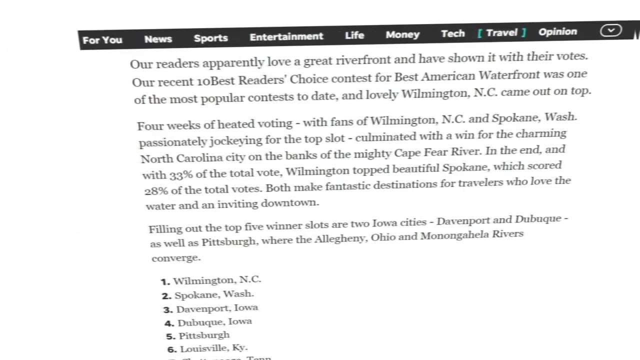 lows of our country's history. One of the main attractions here is the USS North Carolina battleship that sits majestically at the port. Still on the topic of iconic locations, the port city also attracts its fair share of tourists with the Cape Fear Riverwalk, and is known for. 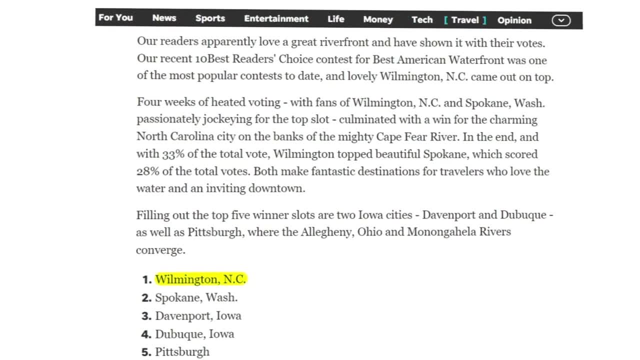 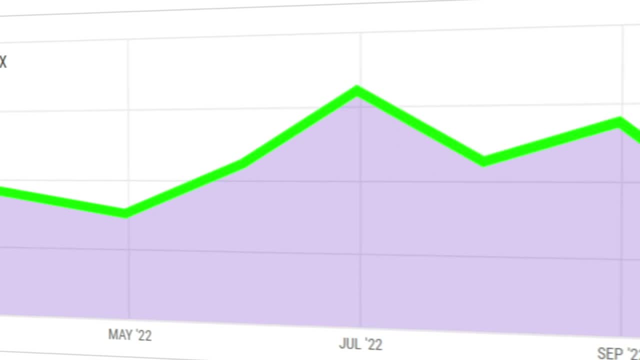 being home to a riverfront that was ranked best American riverfront in USA. Today, Away from the aesthetics and landmarks of the city, Wilmington has an unemployment rate of three percent, which is both lower than the state and national average. In addition, the port city has an 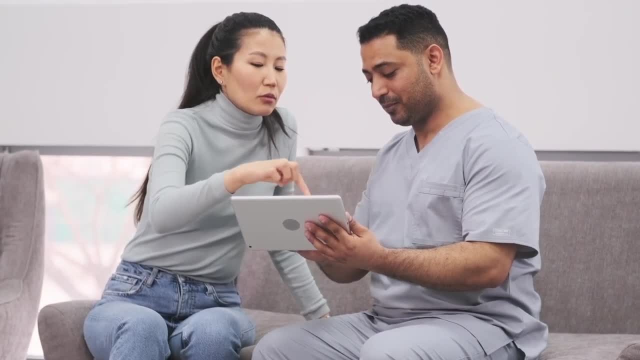 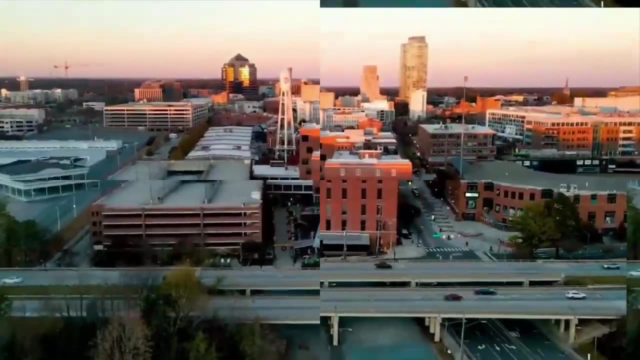 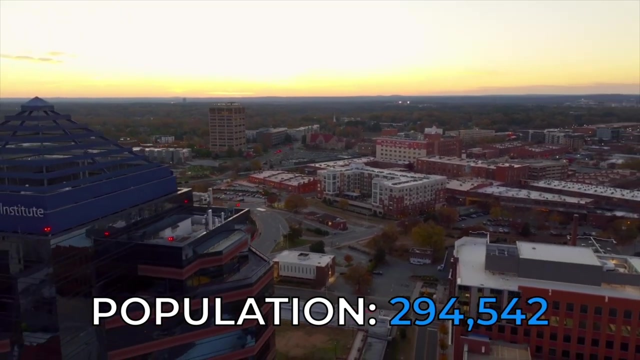 outstanding health care system that puts it among the top 100 healthiest cities in the country. 8. Durham- The big city of Durham is located in the county seat of Durham and has a population of about 294,542 residents and a total land area of 112.2 square miles. 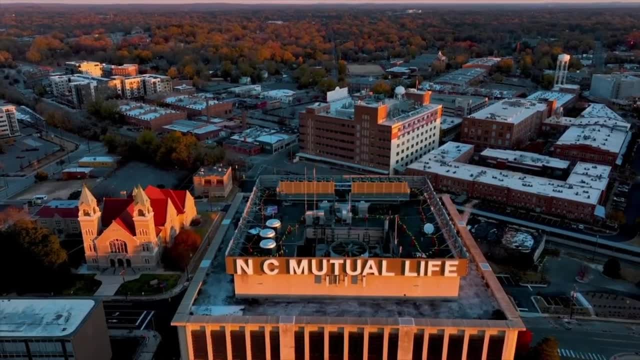 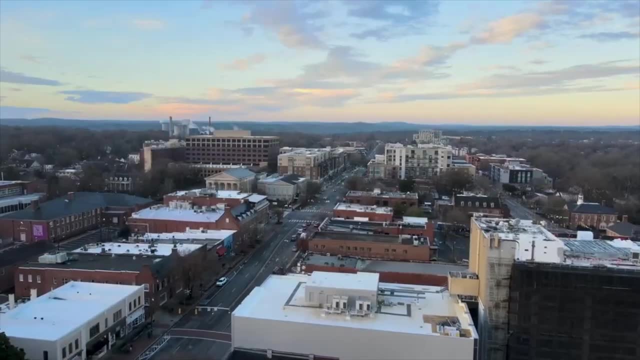 8. Durham. The big city of Durham is located in the county seat of Durham and has a population of about 294,542.. The city is ahead of most other North Carolina cities and is a part of the trio of research partners, with the other two members being the state capital of Raleigh and the thriving town. 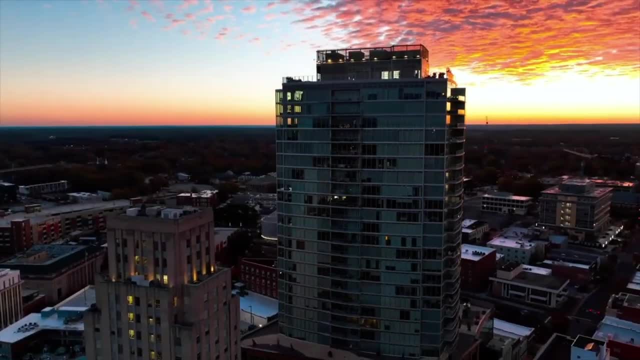 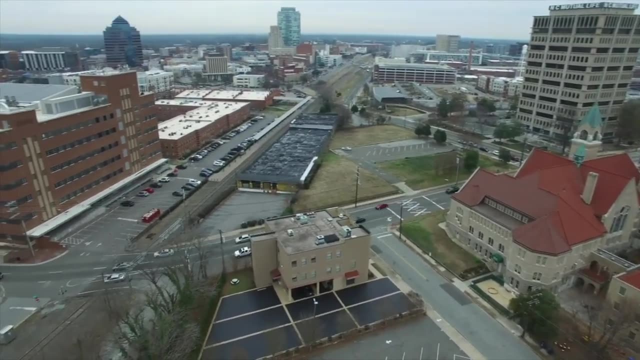 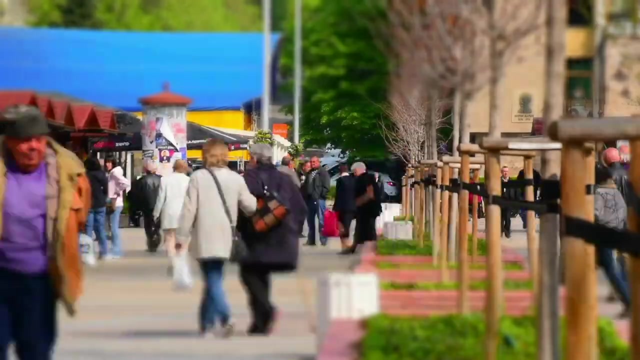 of Chapel Hill. As one would expect, this strategic partnership contributes to the city's strong economy. Durham gives its residents and tourists a sense of belonging, despite its size, and draws them in with its beautiful green spaces, museums and friendly locals. One of the many 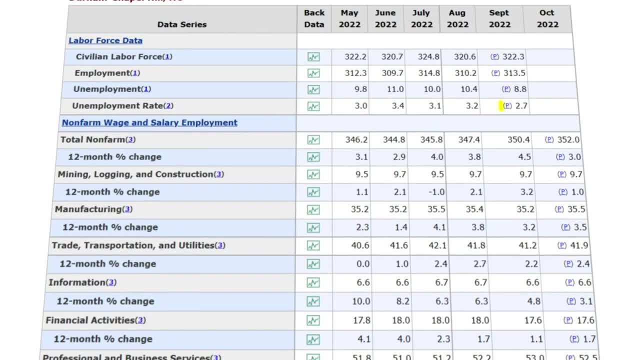 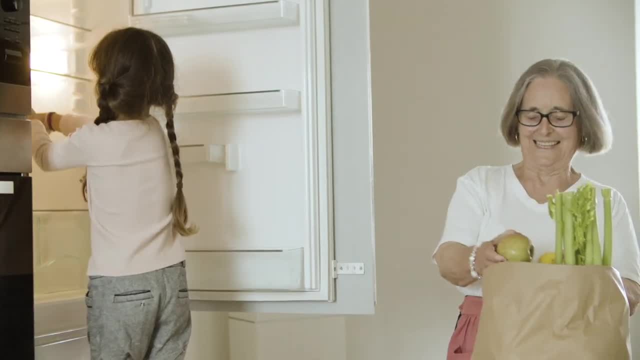 perks that come with living in the Bull City is that it has an unemployment rate that is considerably lower than the national average. The cost of living here is also lower than the national average. With all these in mind, it's easy to see why Durham is tagged as one of the 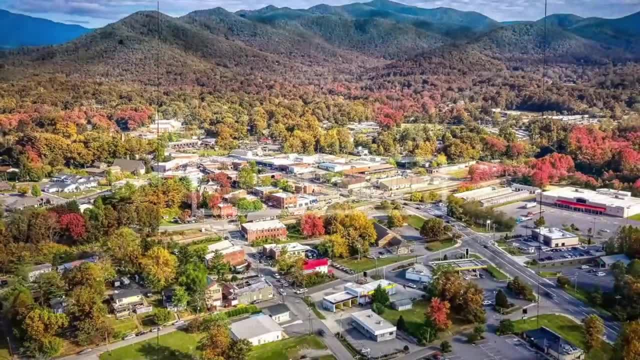 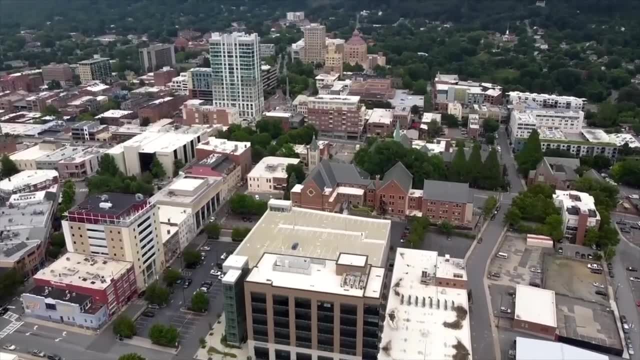 best places to live in North Carolina. 7. Asheville, Located in the county seat of Buncombe, is the largest city in western North Carolina. Asheville- Asheville is called land in the state of Durham. It's the largest city in the state of Durham. It's the largest city in the 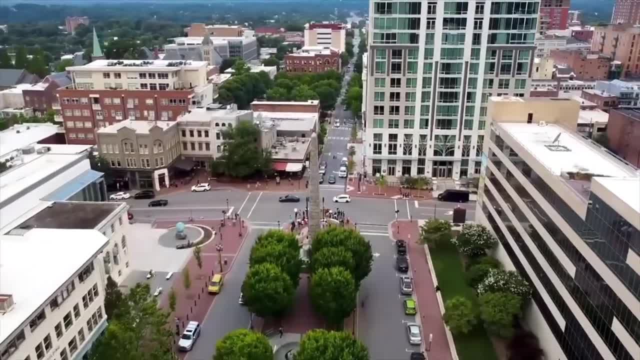 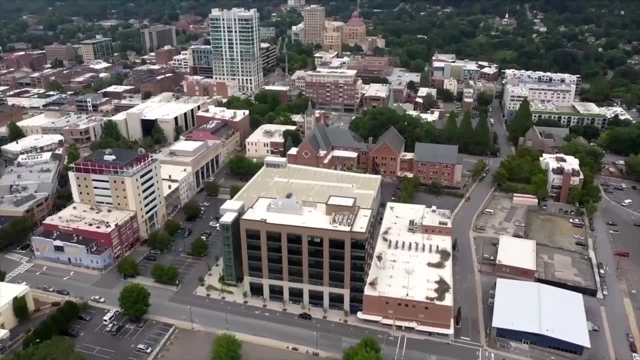 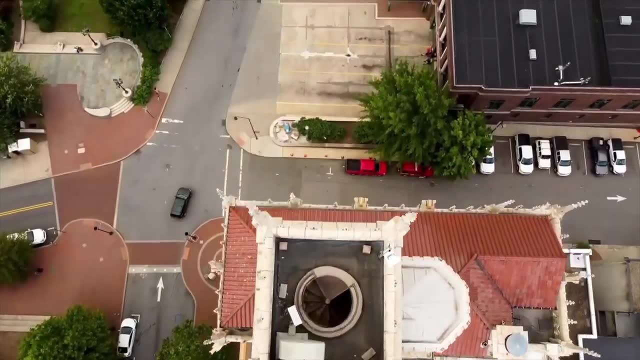 sky for many reasons, and one of them is that it is indeed a paradise-like place to be complete with fine tropical weather. Currently, the land in the sky has a population of about 96,829 and a land area of about 45.6 square miles, One of the many reasons why Asheville 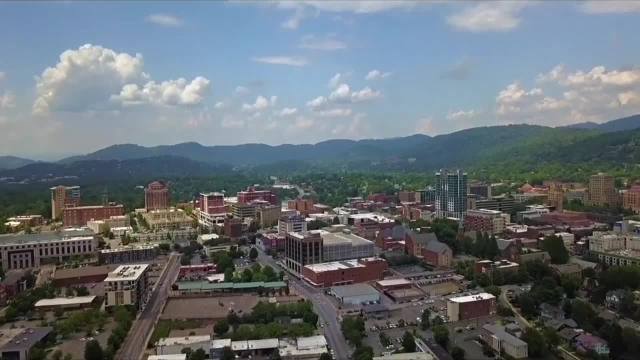 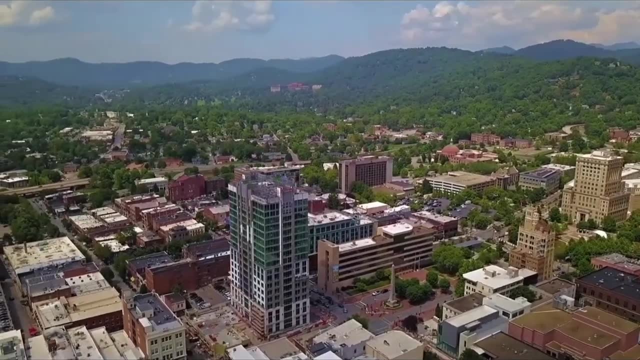 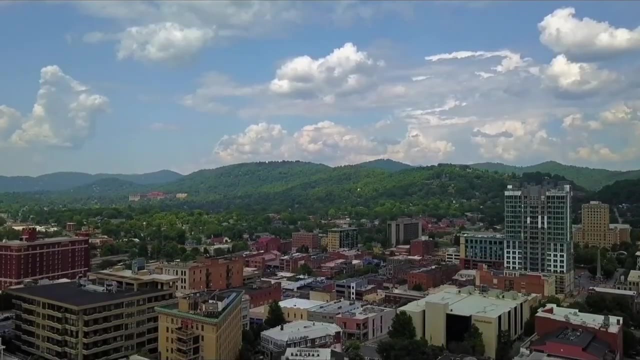 is one of the best places to live in the state of North Carolina is the city's proximity to great outdoors. The Blue Ridge Mountains make a beautiful backdrop for the residents of Asheville, and that is just one of the many attractions that earned it the alias. the Paris of the South, Away from the beauty of the city and the friendly 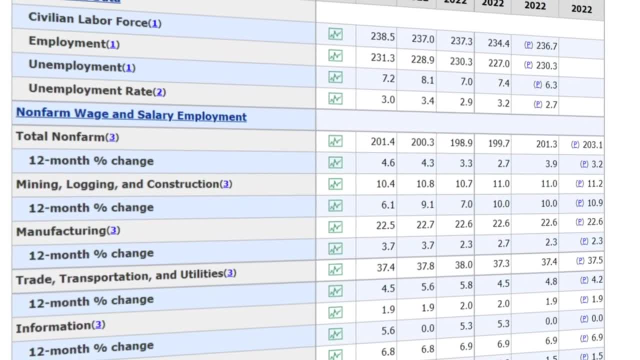 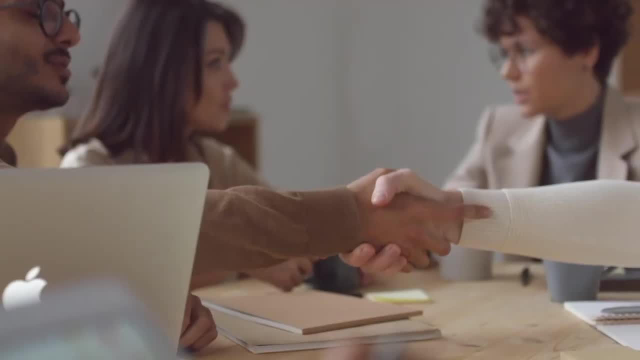 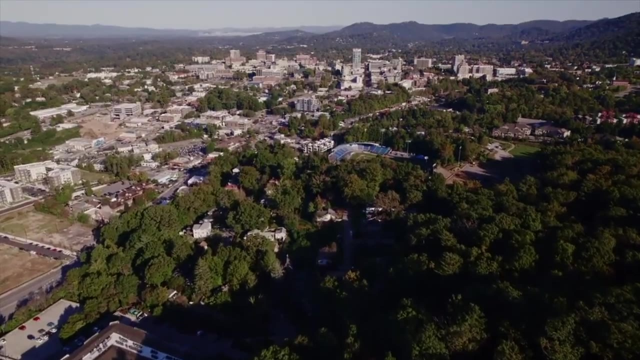 nature of its residents. the numbers are also pretty impressive. The unemployment rate here is almost half the national average, which means you will have no problem securing a job to help pay the bills. That and the fact that Asheville has the fifth best education system. 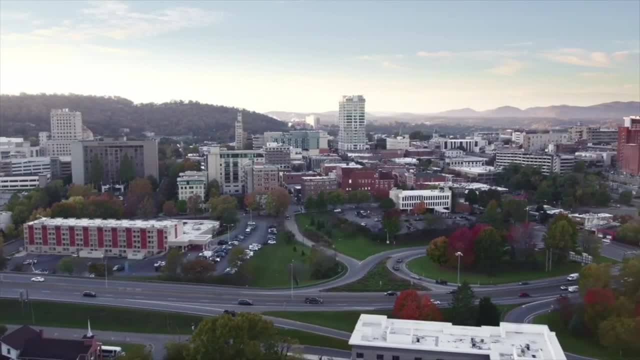 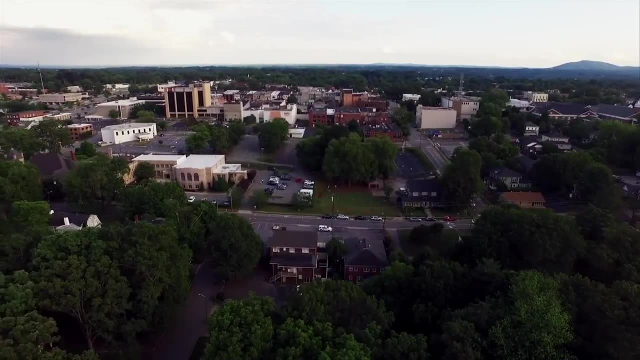 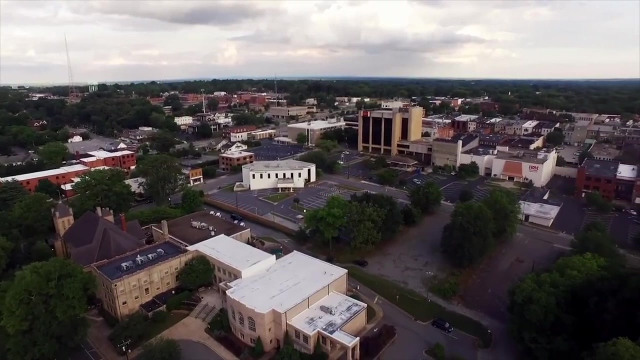 in the state makes it the ideal place to live and raise a family. 6. Hickory: Living in the city of Hickory means you have everything ranging from a moderate climate to sweeping mountain views. Hickory is located in Catawba County, just northwest of Charlotte. 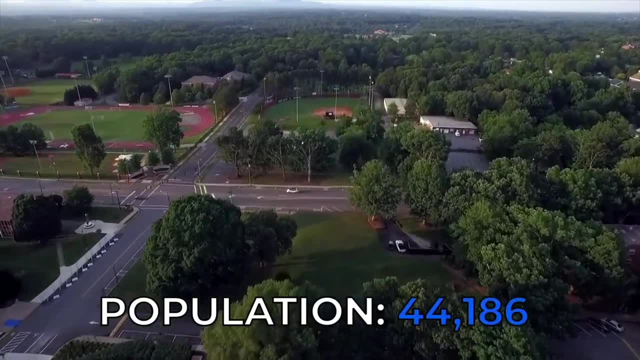 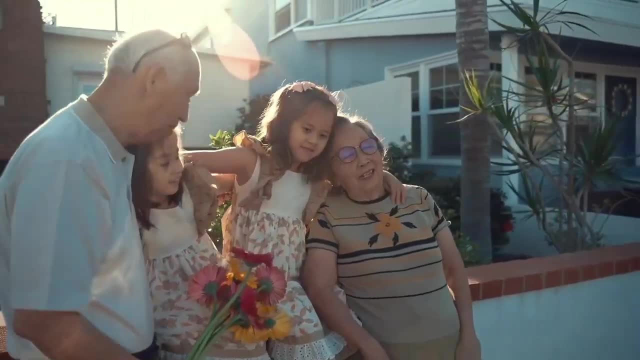 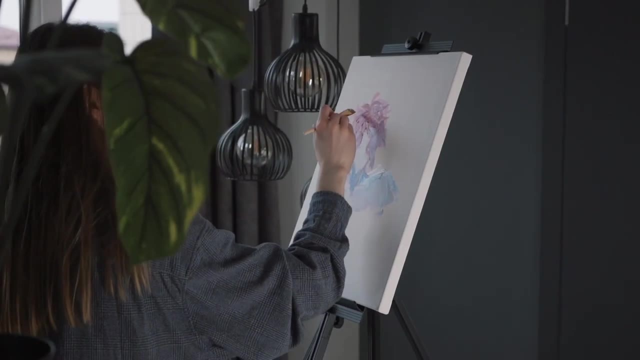 and the city has a population of about 44,186 residents, with a land area of 29.6 square miles. In recent years, Hickory has become not just a haven for families and retirees, but also home to young professionals. The city boasts of strong artistic roots, so it's no surprise that there are masterpiece. 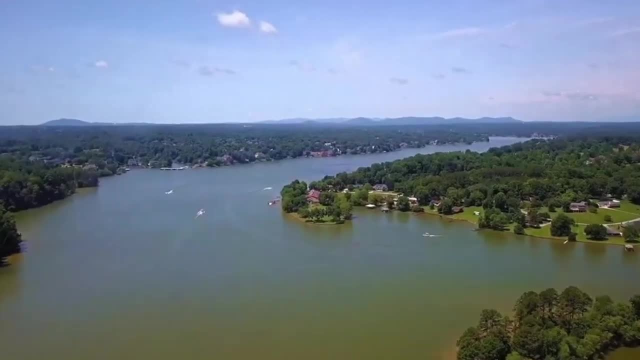 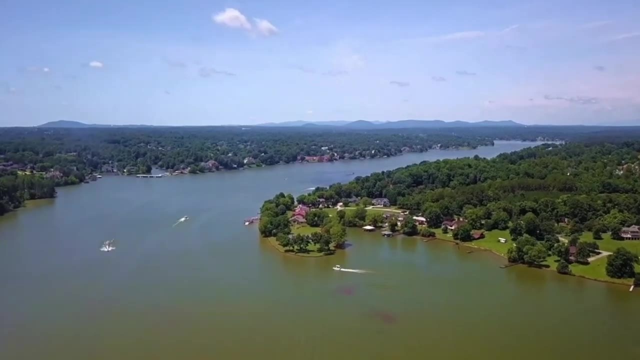 sculptures from local artists on display. For adventure lovers, especially seafarers, Hickory has its own Lake Hickory, which is the largest man-made reservoir in the world. The lake rests on the east side of the well-known Carolina Catawba River, which runs from Lake Hickory to Lake Hickory. Hickory is the largest. 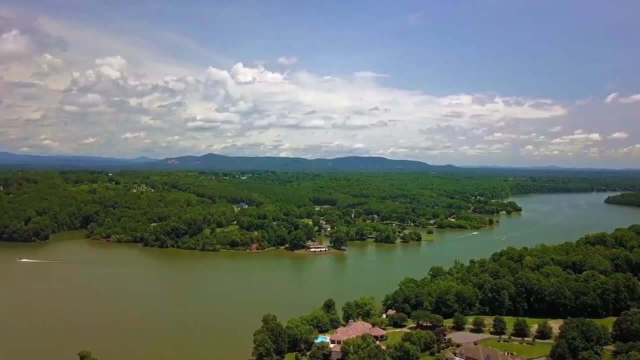 man-made reservoir in the world. The lake rests on the east side of the well-known Carolina Catawba River, which runs from Lake Hickory to Lake Hickory. The lake runs for about 225 miles through both North and South Carolina, Although Hickory 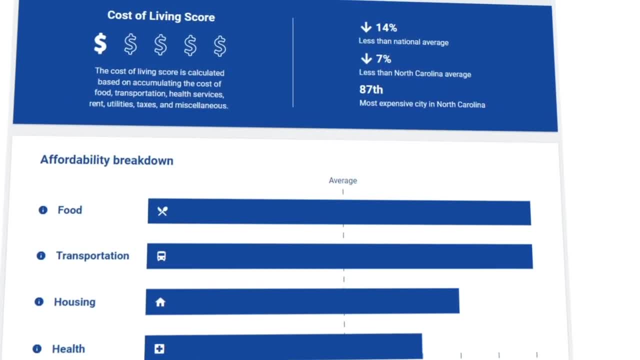 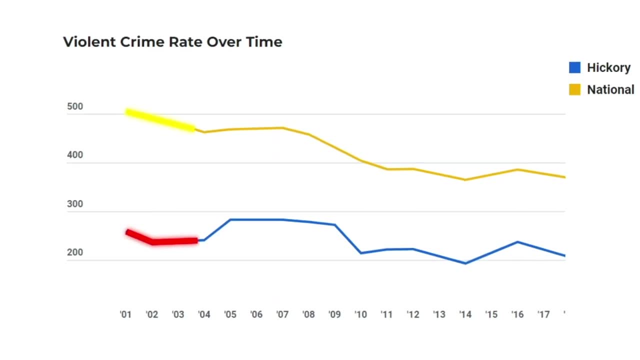 is not the cheapest North Carolina city. the cost of living here is still 14 percent less than the national average and 7 percent less than the state average. The city also has a lower crime rate than the country's average. By many standards, Hickory shows itself as 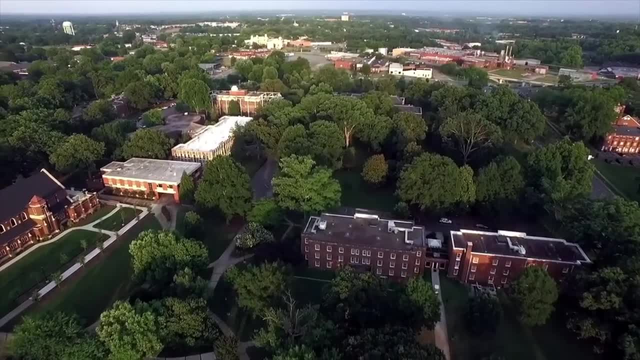 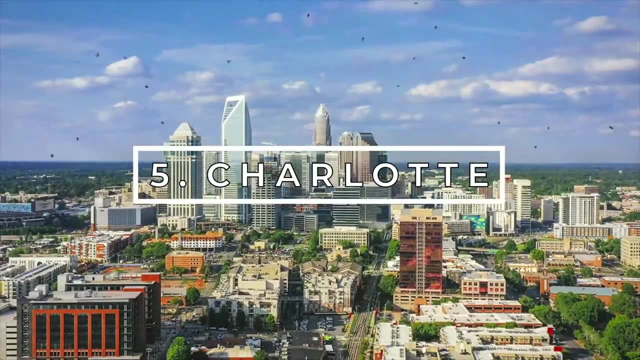 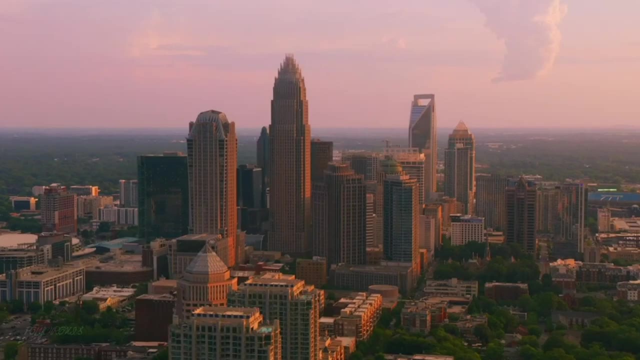 one of the best places to live in North Carolina by offering such a high quality of living at a relatively low cost. 5. Charlotte. Charlotte is a charming yet sprawling Southern city located in the Piedmont region in the county seat of Mecklenburg. The pleasant urban city is one of the most populated cities. 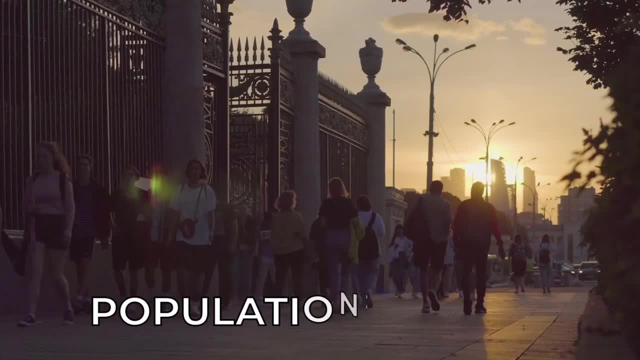 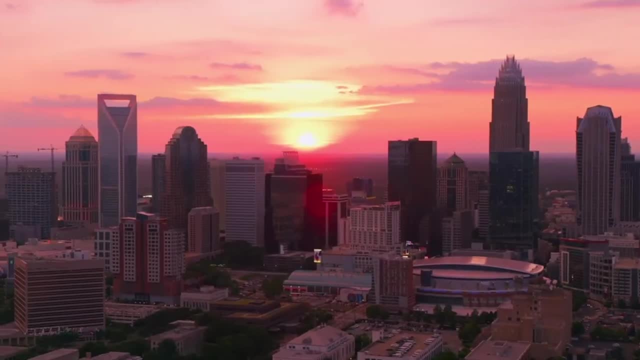 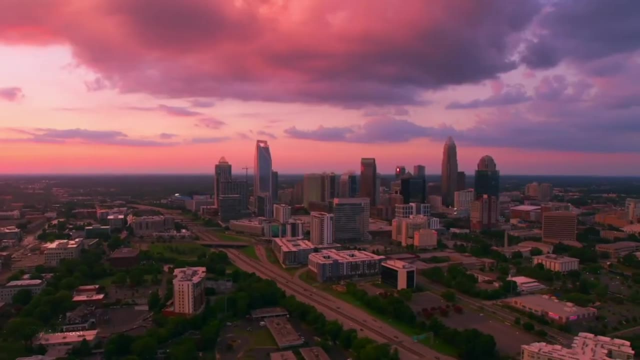 in the state. with a population of around 903,211 residents and a total land area of 307.2 square miles, Charlotte has a strong economy that stems from it being the second-largest banking center in the whole country. This status contributes significantly to the obvious. 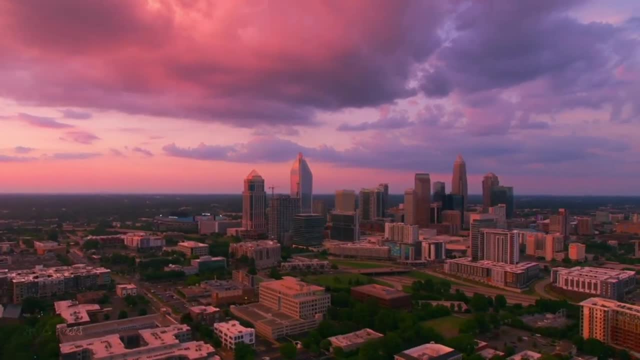 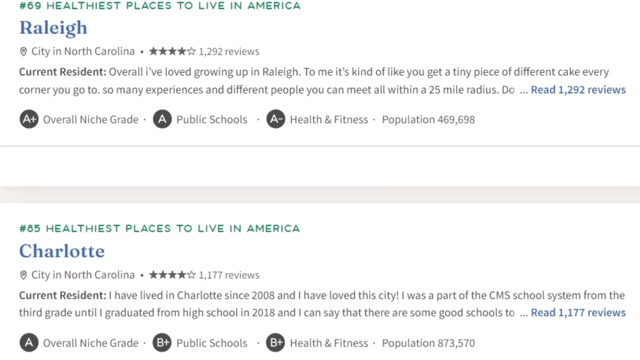 population growth of the city and its development into one of the best places to live in North Carolina. Charlotte also has one of the best health care systems in the state and is also ranked among the top 100 healthiest places in the country, Although Charlotte is one. 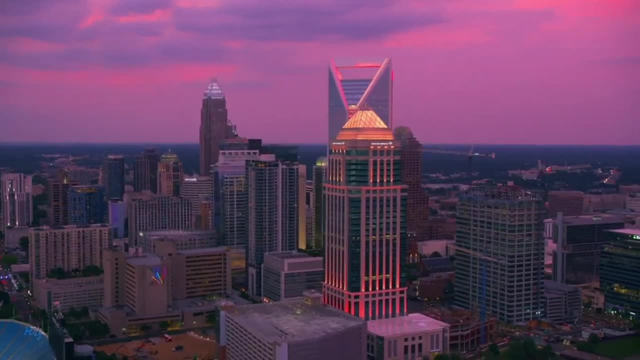 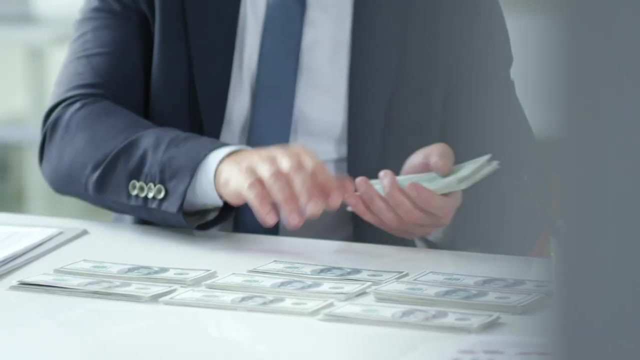 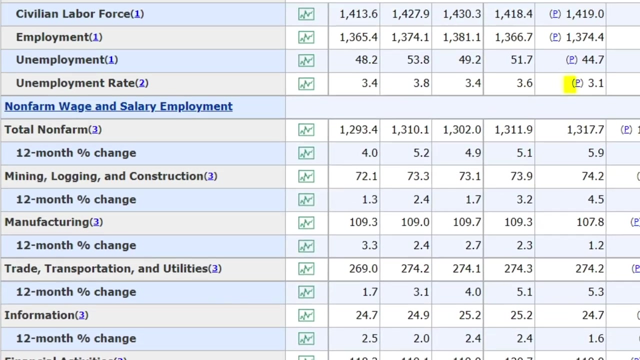 of the fastest growing cities. the cost of living is balanced with the state average and less than the national average. So while you may not be saving as much as you would like, you will definitely not have to break the bank to pay bills. The rate of unemployment here is also less than the national. 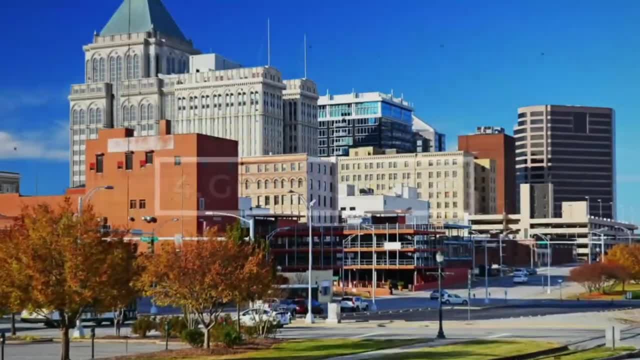 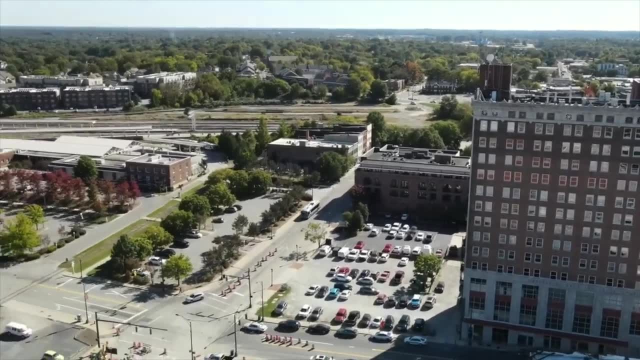 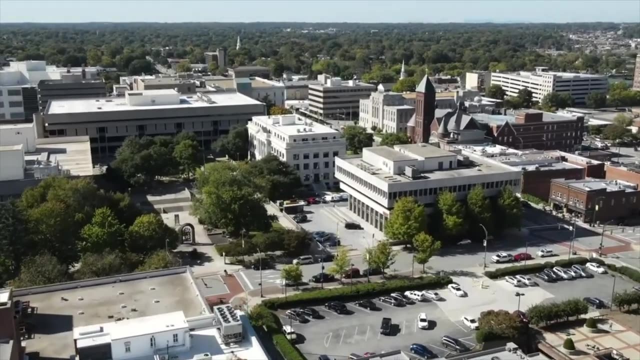 average, which is always a plus 4.. Greensboro Being the third most populous city in the state of North Carolina, Greensboro is one of those places that is big enough to have everything you could possibly need, and yet small enough for you to bump into someone you know. every now and then, The gate's. 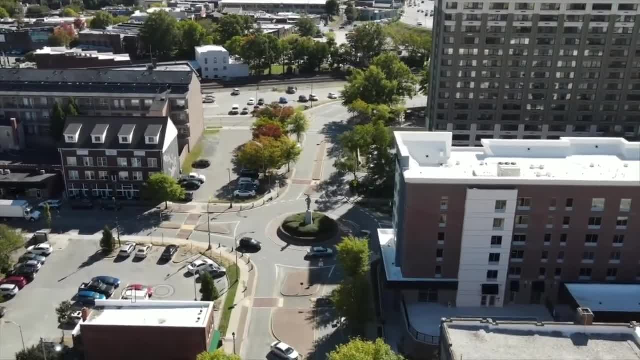 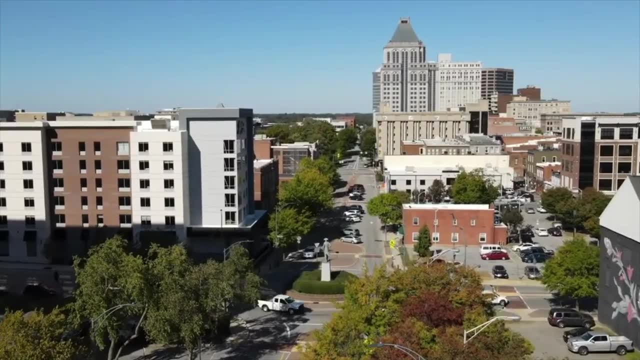 city sits on the county seat of Guilford and has a population of about 304,909 residents. If you ask any of those thousands of people, most of them would say that they simply love living in Greensboro and that there's no place like it. 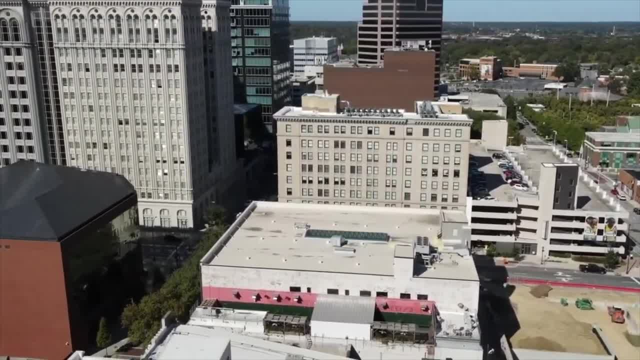 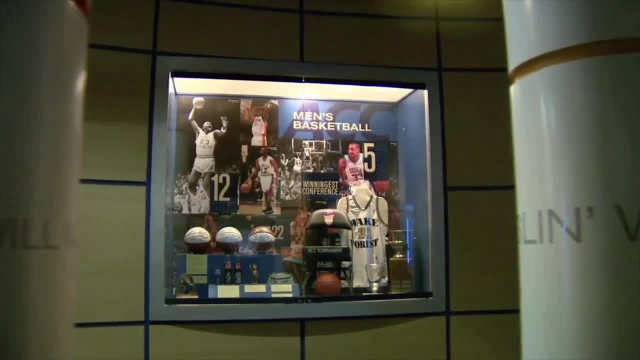 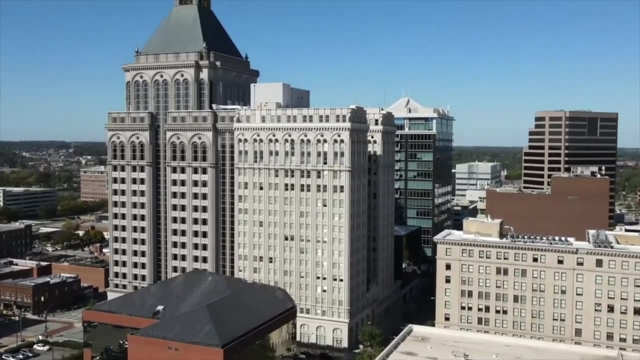 For a not-so-big city, Greensboro is bursting with attractions for residents and tourists. Places like the ACC Hall of Champions, the History Museum and the Coliseum Complex offer a captivating and equally-enhancing experience. 5. Greenville: For those looking for a lively downtown, downtown Greensboro has you covered, Needless. 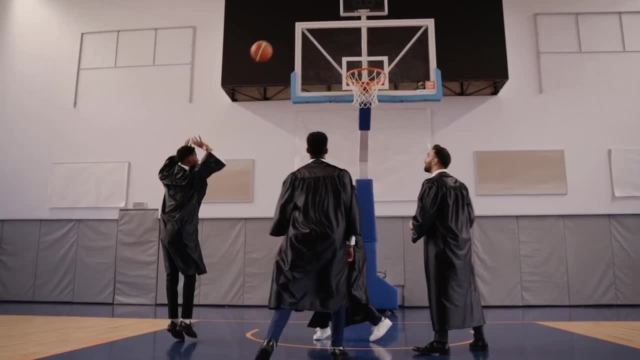 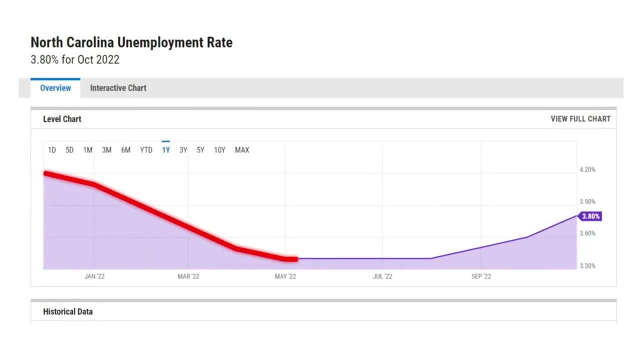 to say. the gate city is a good fit for all kinds of people, ranging from students to young professionals and families. Greensboro has an unemployment rate that is slightly less than the national average. That, along with its strong economy, thriving arts and cultural. 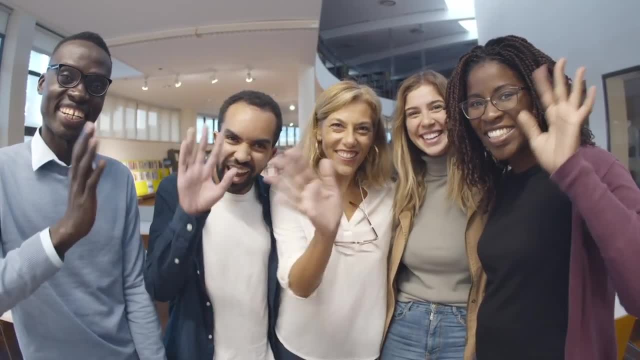 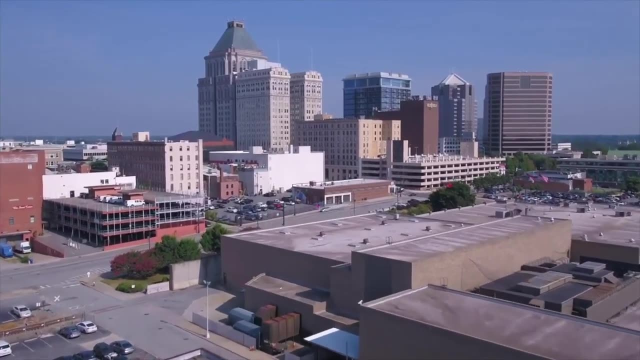 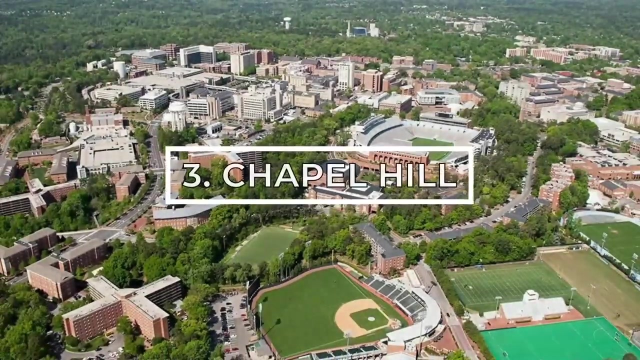 scene and friendly neighborhoods make this city not just one of the best places to live in this big state, but also the whole country. A little fun fact about Greensboro is that at least 19 US presidents have visited the city. 3. Chapel Hill. 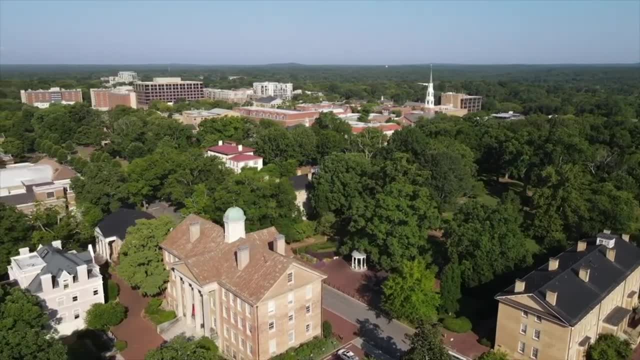 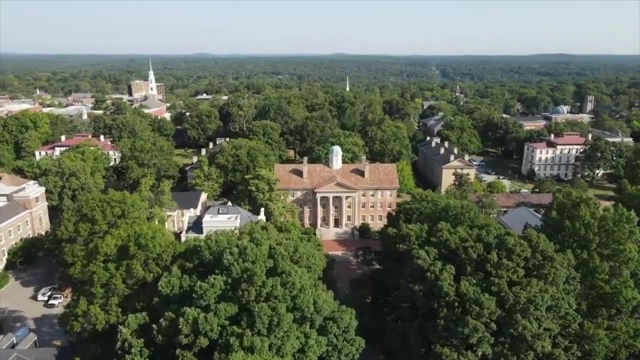 The small town of Chapel Hill is located in Orange, Durham and Chatham counties. It has a population of about 62,906 people and a total land area of 21.5 square miles. Chapel Hill is also one of the most populous cities in the country. It's home to the University of. 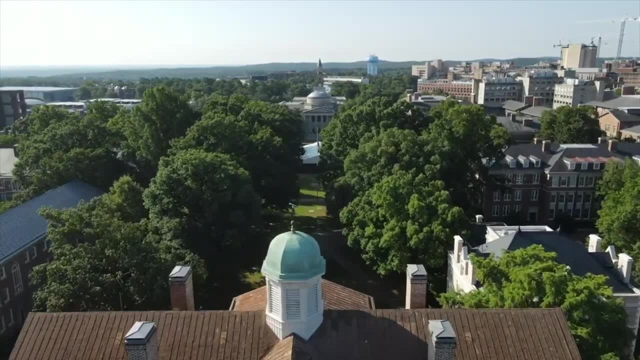 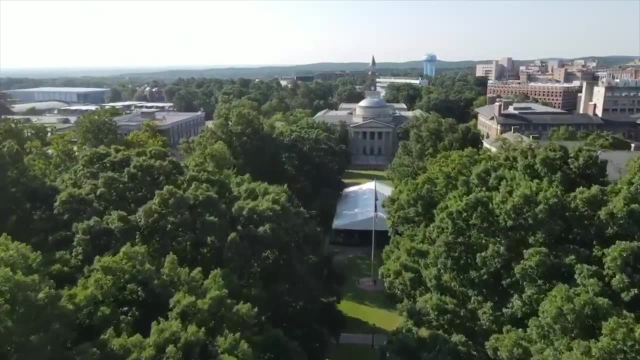 also one of three towns, with the other two being Raleigh and Durham, that make up the Research Triangle, which got its name due to the three major research universities in these cities. Chapel Hill gives its residents a sense of community with its small-town charm. 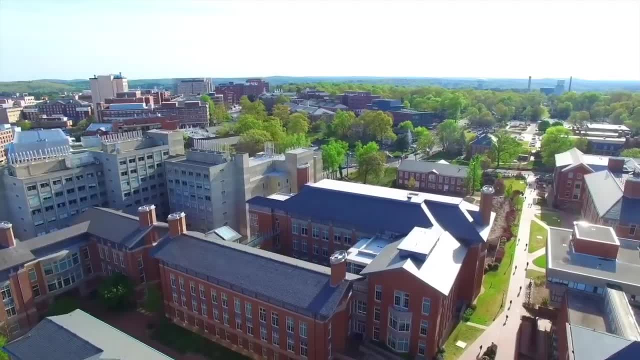 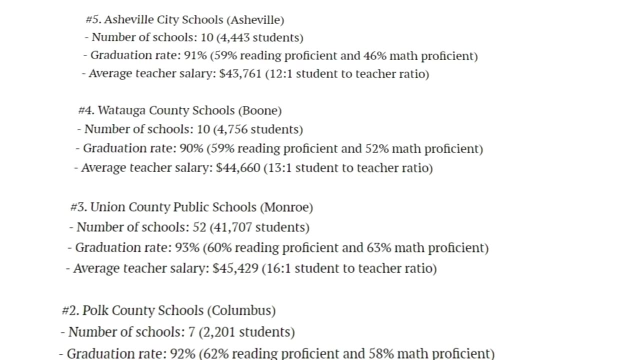 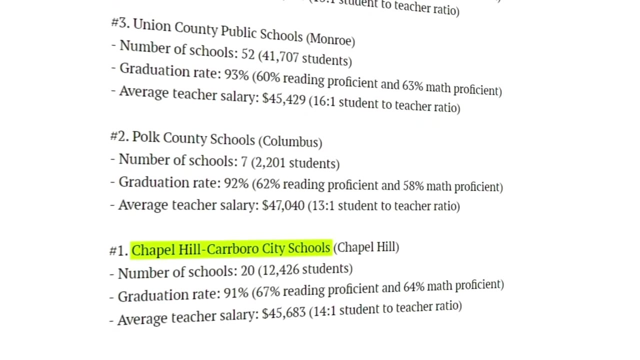 beautiful green spaces, museums, a big artistic community and distinct seasons that offer the best of summer, winter, autumn and spring. Away from the seemingly perfect weather and the aesthetics, Chapel Hill boasts an educational system that is ranked as the best in the state. 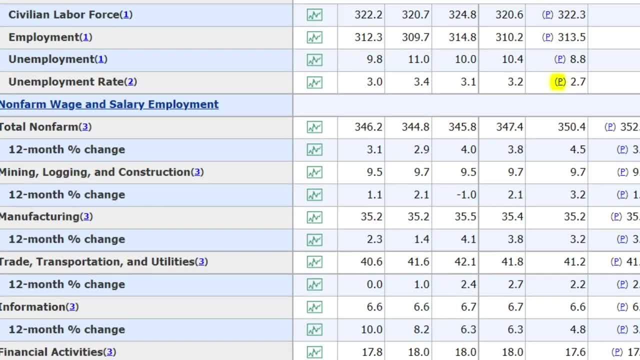 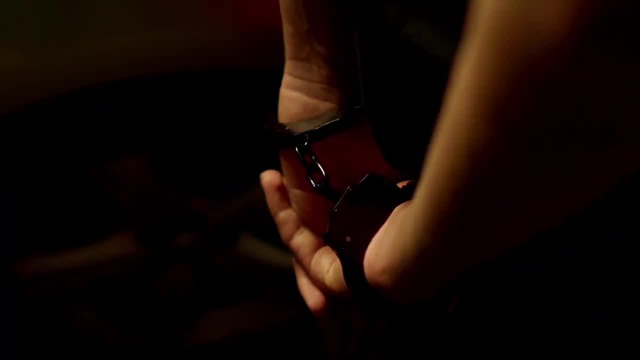 The unemployment rate here is also considerably lower than the national average, so paying your bills shouldn't be that much of an issue. Where safety is concerned, Chapel Hill has a crime rate that sits below the national average, making it one of the safest places to live in North Carolina. 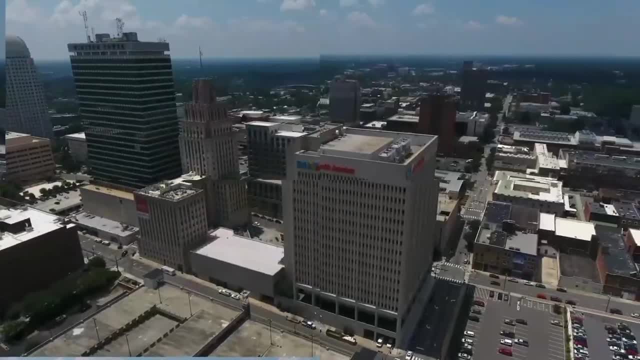 2. Winston-Salem. Not many cities can boast of having two names, and the one that's most popular is the one that's the most popular. 2. Winston-Salem. Not many cities can boast of having two names, and the one that's most popular is the one that's the most popular. The ones that do have something special to show for it. Winston-Salem, in the Forsyth County of North Carolina, is one of such cities, and it is one of the best places to live in North Carolina for a host of reasons. The Twin City is the fifth largest city in the state, with a total land area of 132.6 square. 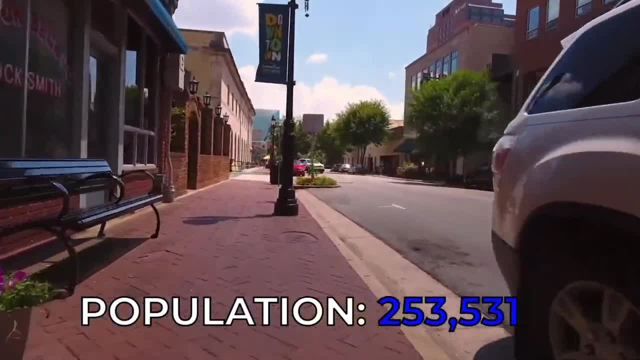 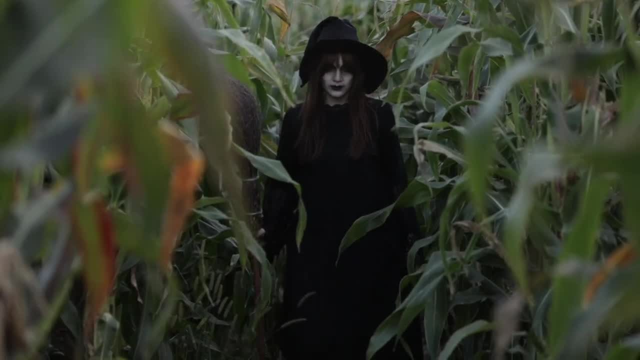 miles and a population of around 253,531 residents. Just like the city of Salem was known for its witchcraft, Chapel Hill is one of the most popular cities in North Carolina. Back in the day, Winston-Salem is known for its art. The city is home to the Rinalda House Museum.